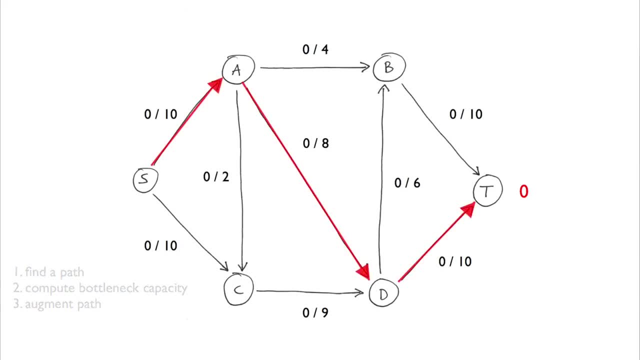 forward or non-empty and backward. Let's choose the following path first. The bottleneck capacity is A to D, a value of 8. We'll augment all edges with this value. Also, note that each node must remain in equilibrium, that is, the flow into the node must equal the 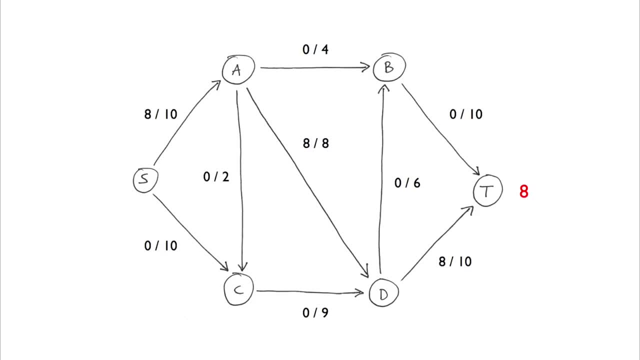 flow out of the node. We're done augmenting, so let's look for our next path. This looks like a good one. The bottleneck capacity is 2 in this case, because edge D T only has a capacity of 2.. Let's update the flow with this value. 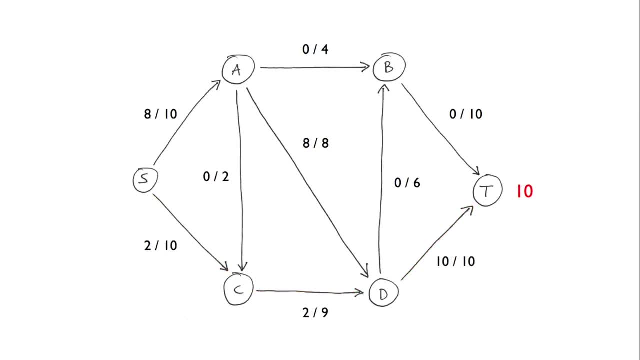 On to the next path. I'm going to specifically choose a path with a backward edge, so you can see how the algorithm works in this case. Note that our path includes going from D to A, even though the edge itself is directed from A to D. 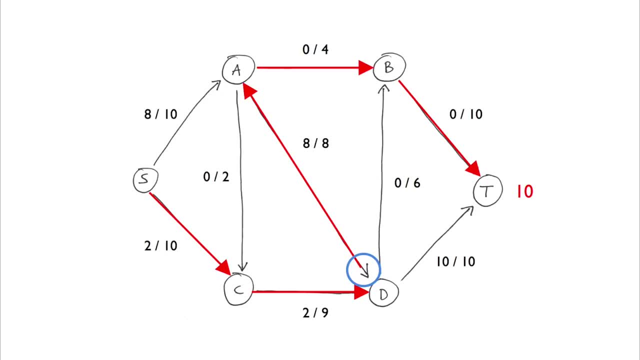 This is what I mean when I say that our path is going from D to A, even though the edge itself is directed from A to D. This is what I mean by a backward edge. Also, notice: D to A is not empty. so if we push 4 units from C to 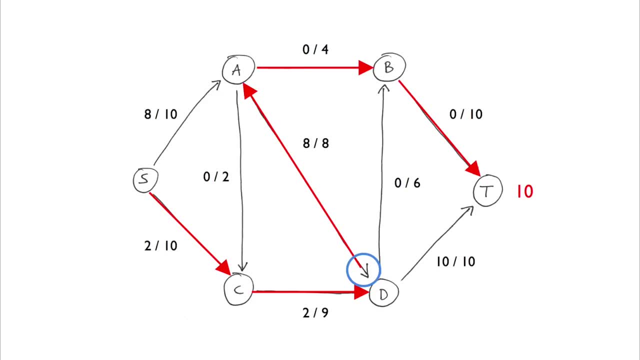 D. we can take away 4 units from D to A, 4 being the bottleneck capacity we receive from edge A, B. This may seem confusing, but just remember that each node must remain in equilibrium. In other words, while we add flow to our forward edges in the path, we take away flow from. 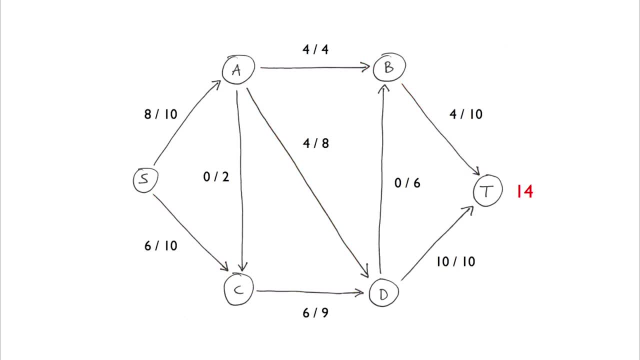 the backward edges. Let's look for another path. This looks like a good one. In this case, edge S to A provides our bottleneck capacity with a value of 2.. We update our flow Again. let's search for a path and augment the flow. 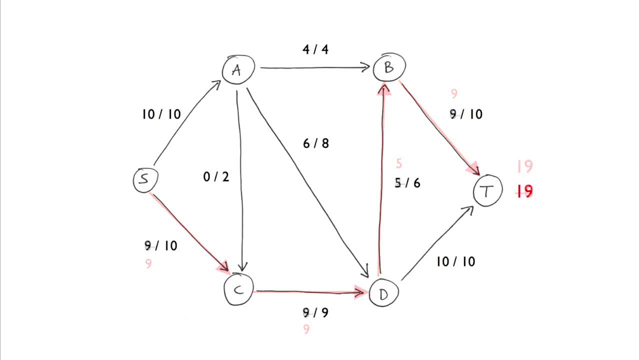 We now have a flow value of 19.. One more time, let's search for a path. Looking at S to A, we can see the path is full. Now, looking at SC, we notice we have a capacity of 1.. However, the forward edge, CD, is full and the backward edge, CA, is empty.